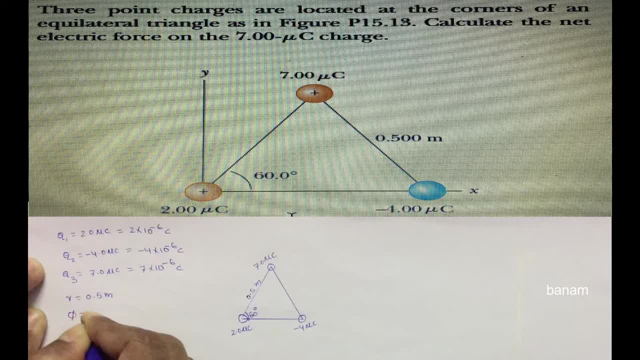 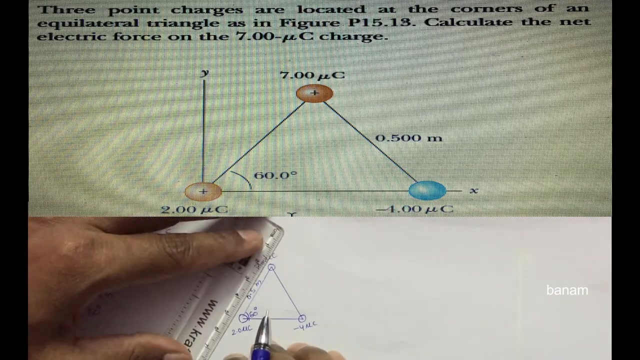 and the angle between them any two charges is 60 degrees. Let us draw the force diagram First of all. we can. we can calculate the force on the 7 microcoulomb charge due to 2 microcoulomb charge and minus 4 micro coulomb charge. The force diagram: the force on the 7 microcoulomb charge. 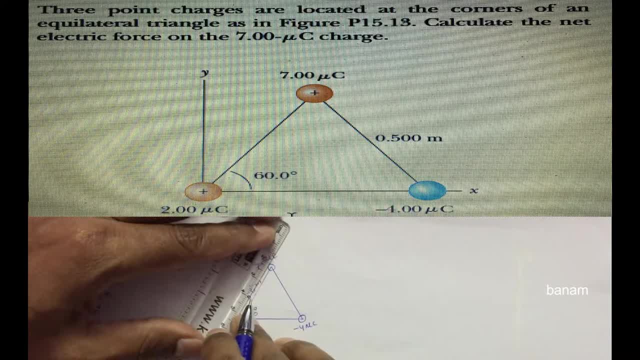 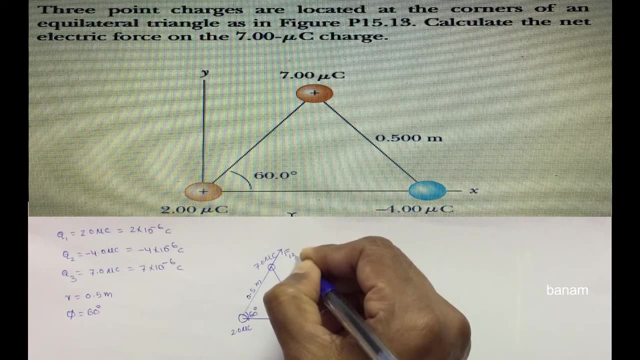 due to 2 microcoulomb charge is along the this direction. The direction is first coordinate of the coordinate system because 2 microcoulomb charge is the positive and minus 4 microcoulomb charge is the negative. The force on the 7 microcoulomb charge is 2 microcoulomb. 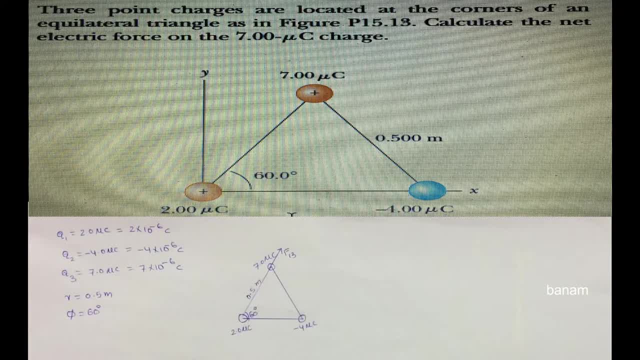 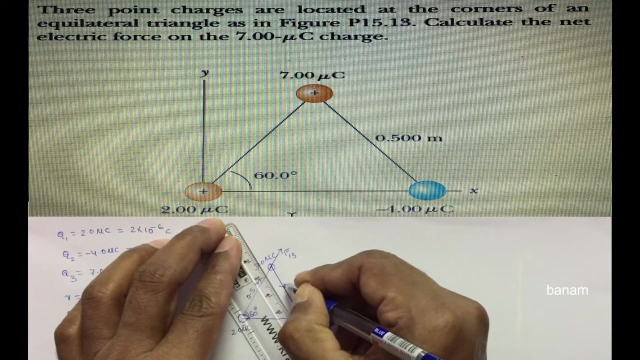 the force always away from the positive charge. so F13 along the first coordinate of the coordinate system and the force on the 7 micro coulomb charge due to minus 4 micro coulomb charge is the direction along the fourth coordinate of the coordinate system, because 4 micro coulomb 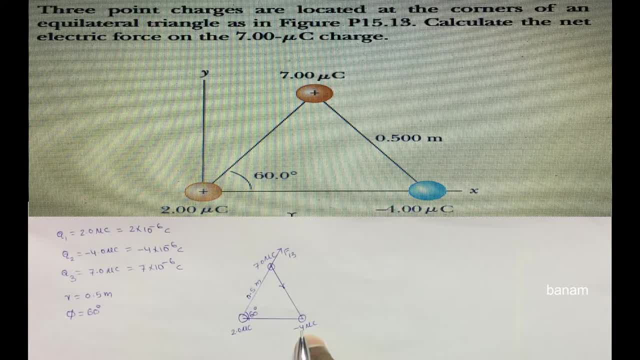 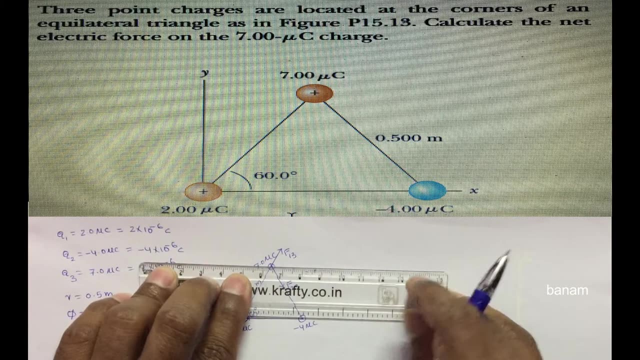 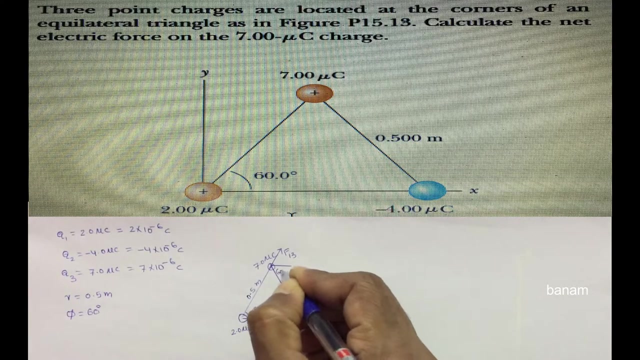 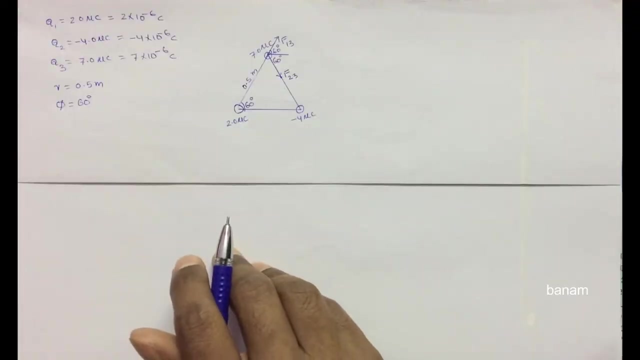 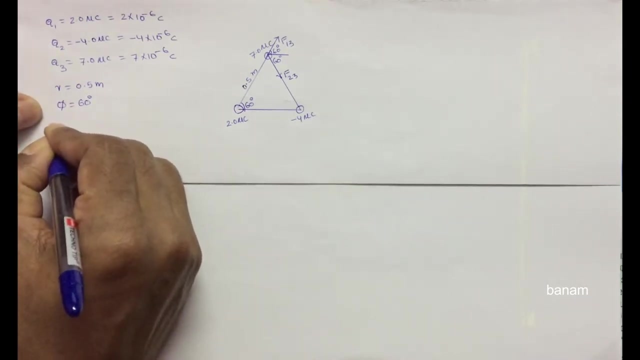 charge is the negative, the force always towards the negative charge. so the force is the F23. the angle between the any two forces from the x-axis is the 60 degrees. this is the 60 degrees and this is a 60 degrees. let us calculate the electrostatic force. the electrostatic force F is equal to K, Q1, Q2 by. 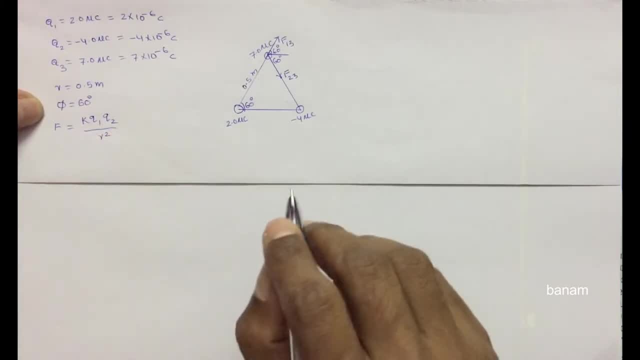 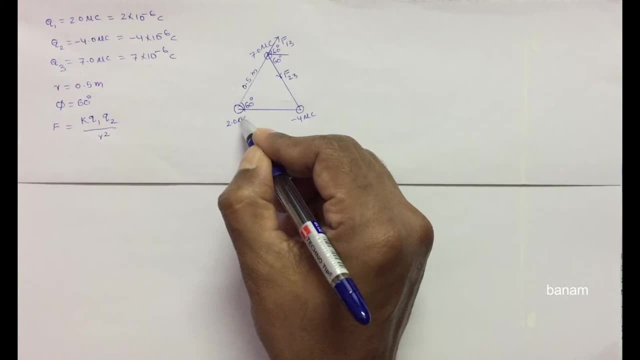 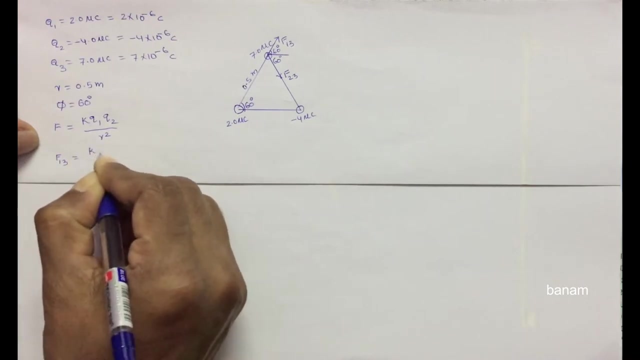 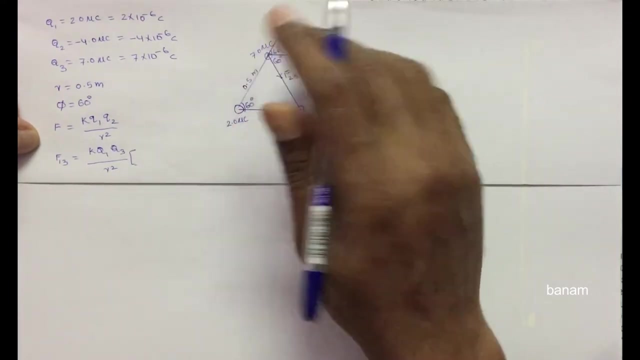 R square. first of all, we can calculate it the. the force on the 7 micro coulomb charge due to 2 micro coulomb charge is F. F 13 is equal to K, Q1, Q3 by R square into the force along the first coordinate of the coordinate system. 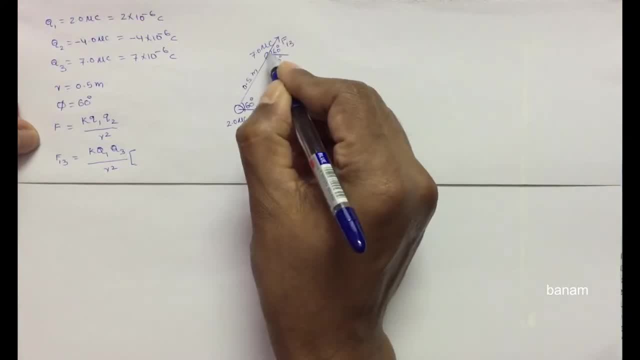 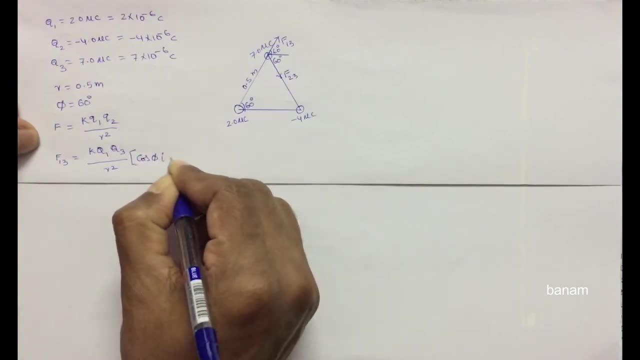 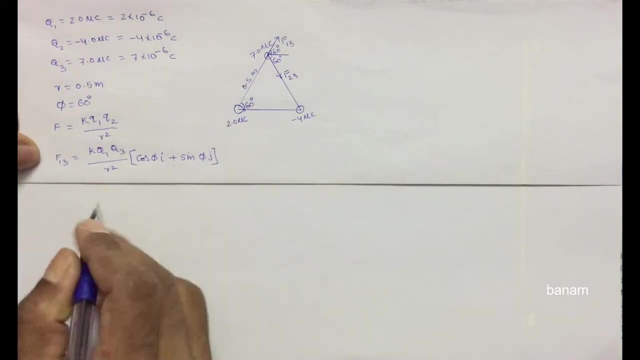 so the x component is positive and y component is the positive. cos Phi I plus sin phi j. Subtract the values F13 is equal to the value of the k is 8.99 x 10 to the power of 9 Newton meter square by Coulomb square x 2 x 10 to the power of minus 6 Coulomb x 7 x. 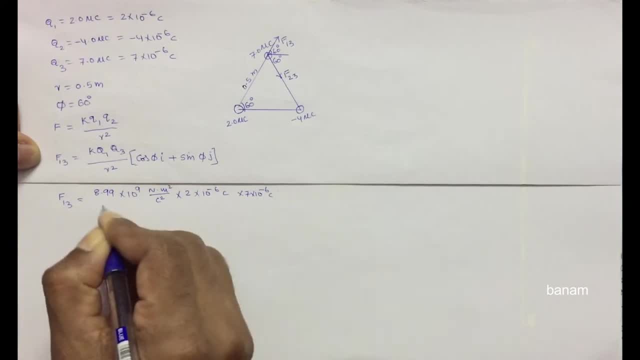 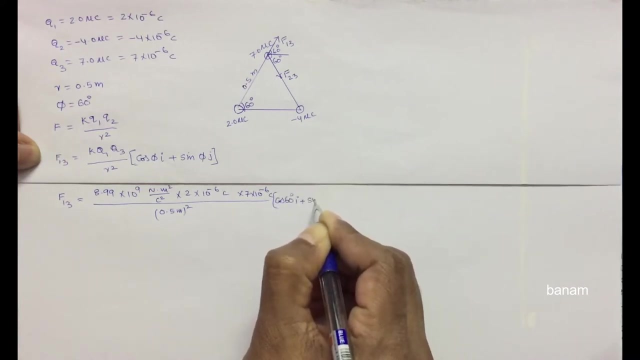 10 to the power of minus 6 whole. by 0.5 meter whole square x, cos 60 degrees I bar plus sin 60 degrees J bar. Calculated, the value F13 is equal to 0.2517 Newton I bar plus. 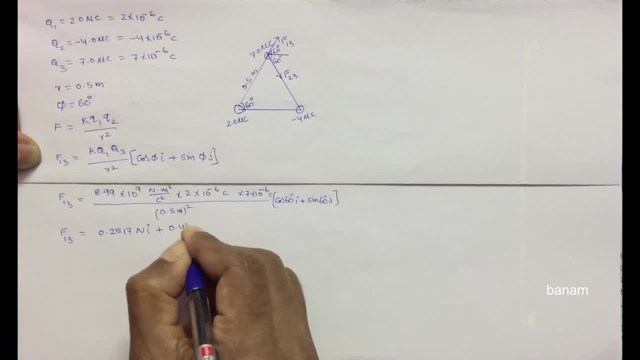 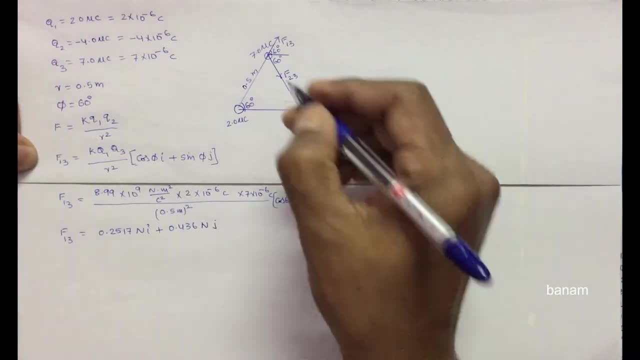 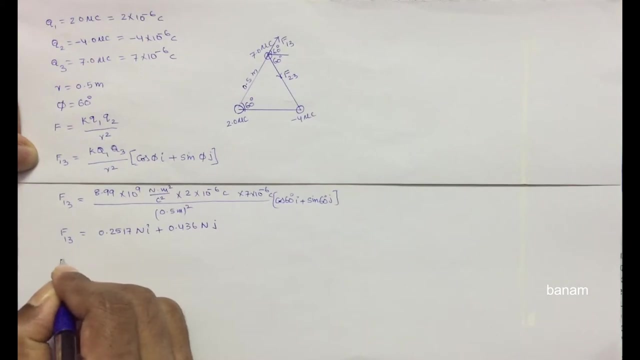 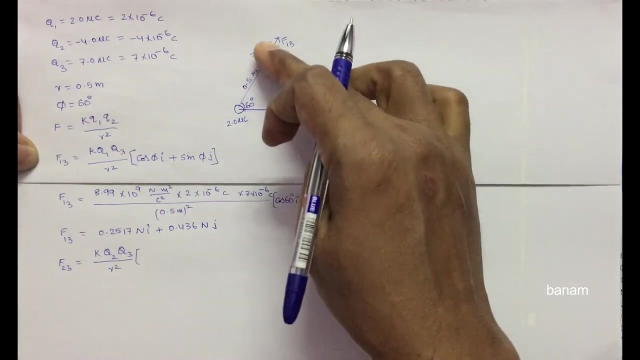 0.436 Newton J bar And calculated the force on the 7 micro Coulomb charge due to minus 4 micro Coulomb charge is: F23 is equal to k, Q2, Q3 by R square into the force along the fourth coordinate. 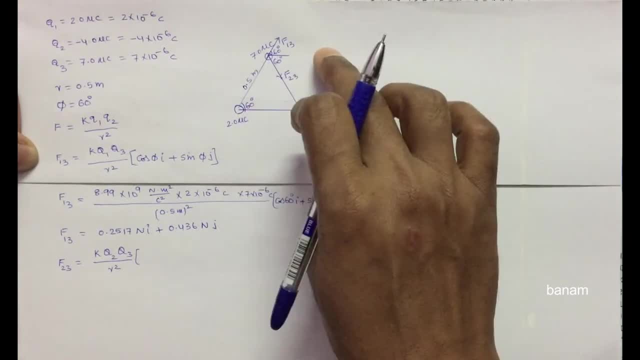 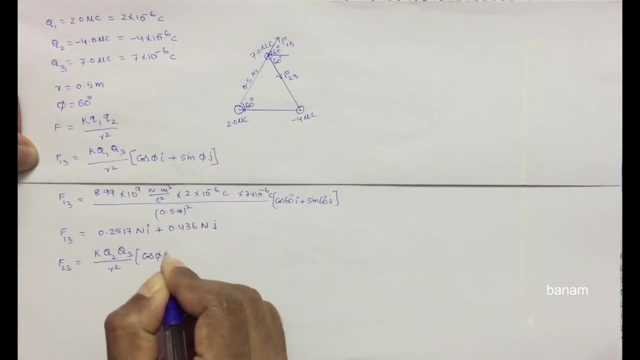 of the coordinate system. So the x component is the positive and y component is the negative. cos phi i minus sin phi j Subtract the values F23 is equal to 8.99 x 10 to the power of 9 Newton meter square by Coulomb square x, 4 x 10 to the power of 9 Newton meter square. 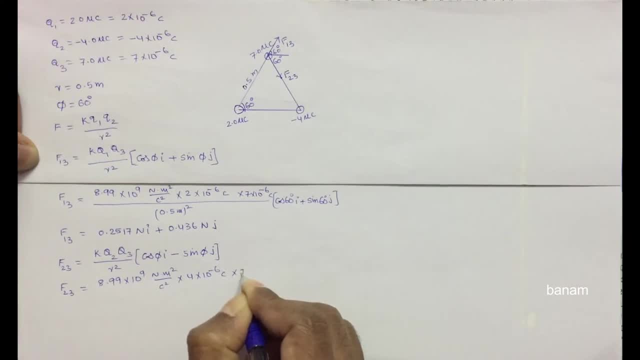 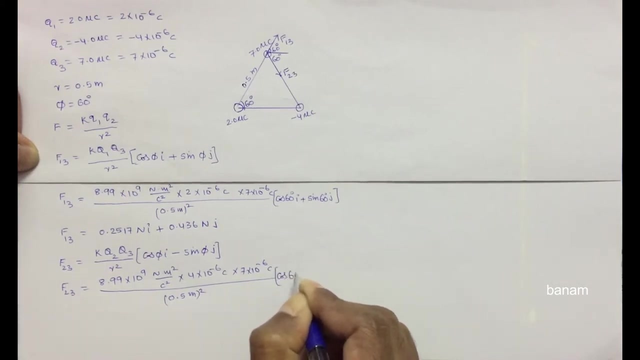 x 7 x 10 to the power of minus 6. Coulomb x 7 x 10 to the power of minus 6. Coulomb whole by 0.5 meter. whole square x, cos 60 degrees. I bar minus sin 60 degrees, J bar Calculated. 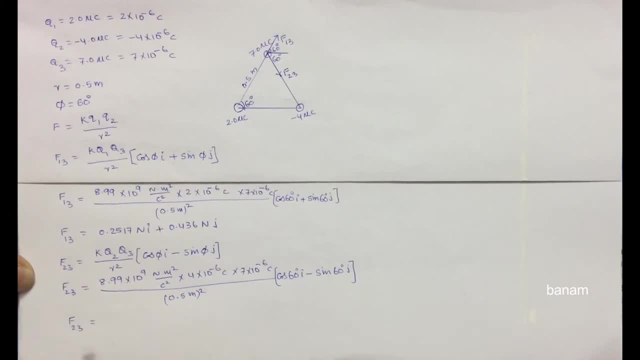 the value F13 is equal to 0.5034 Newton I bar minus 0.872 Newton J bar. The net force on the 7 micro Coulomb charge due to minus 4 micro Coulomb square is 0.5. meter whole square x 10 to the power of 9 Newton meter square x 10 to the power of 9 Newton square x 10 to the power of 9 Newton meter square x 10 to the power of 9 Newton meter square x 10. 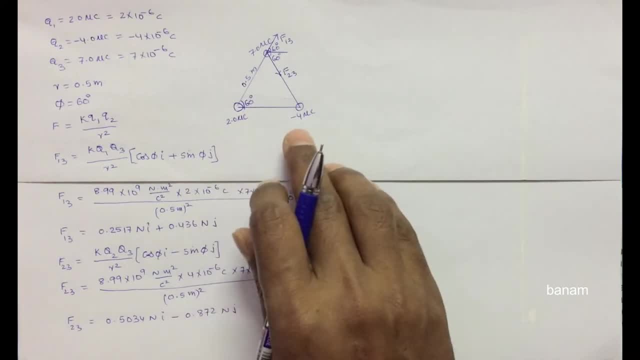 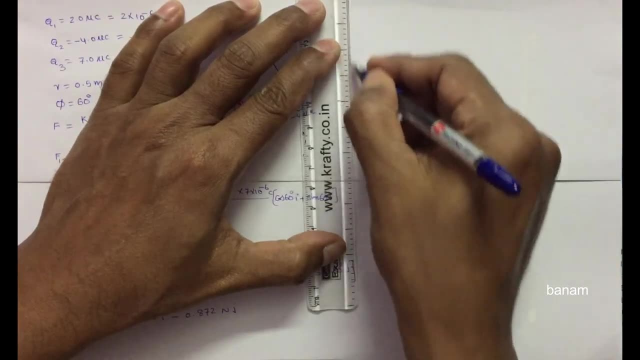 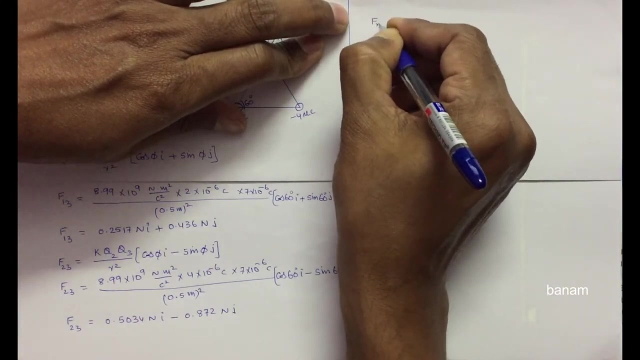 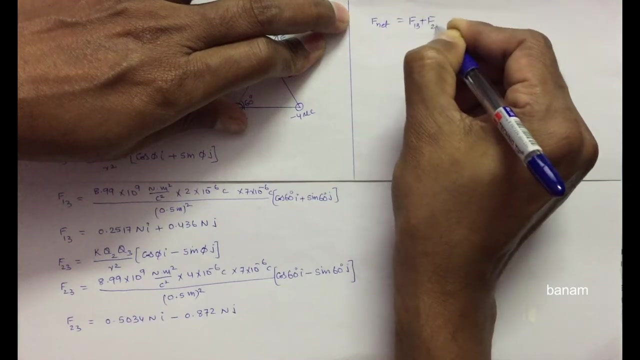 to the power of 9 cm square x 10 to the power of 6 into 3 is F net. F net is equal to sama of the 2 forces. F net is equal to F13 plus F23.. F net is equal to. 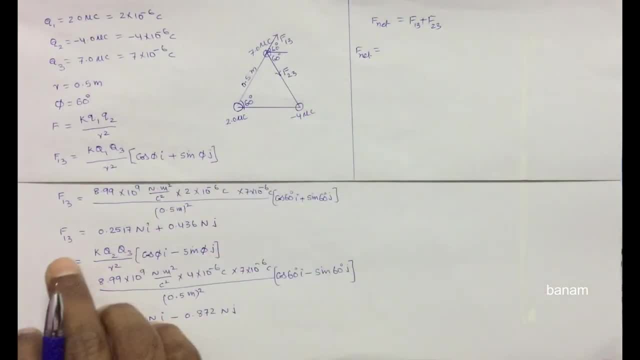 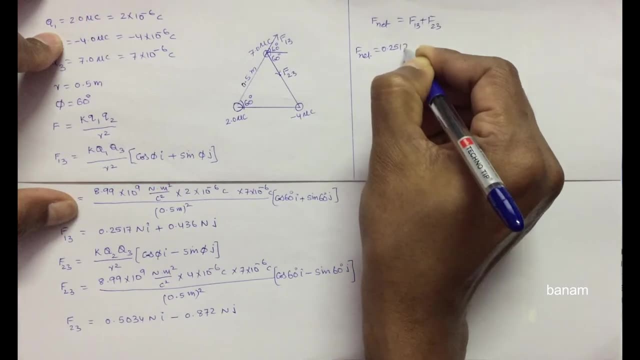 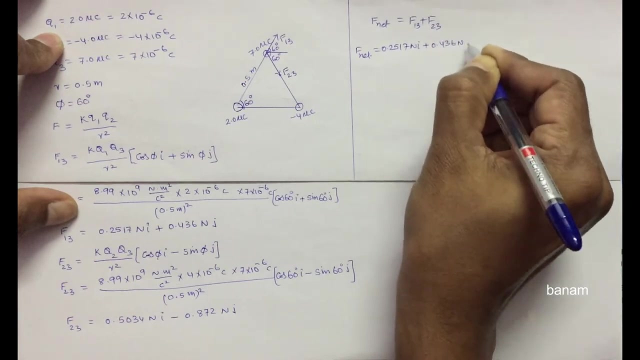 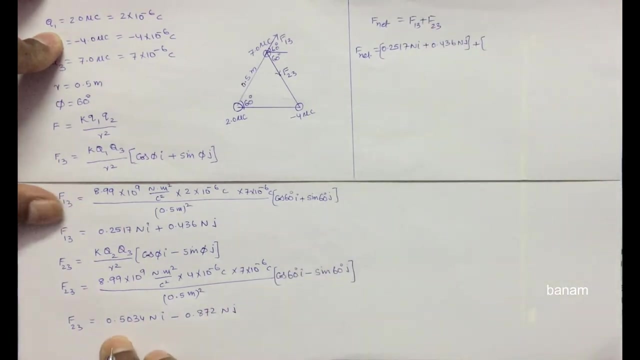 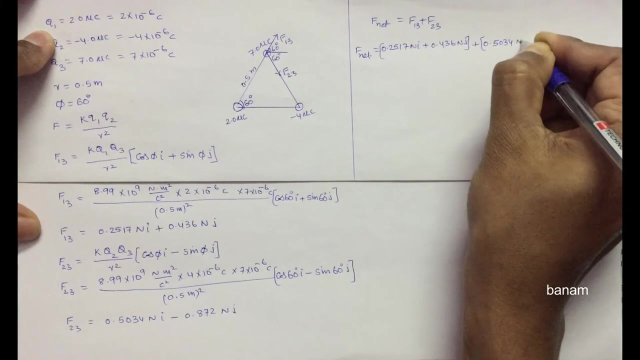 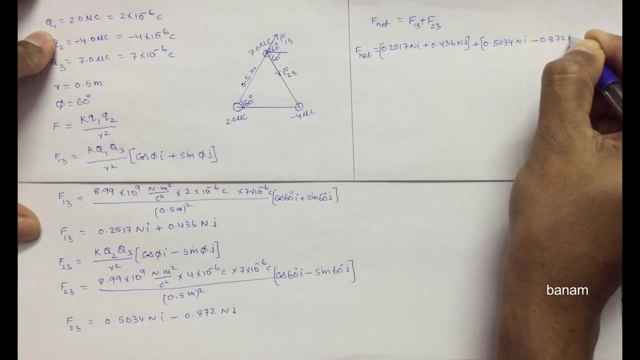 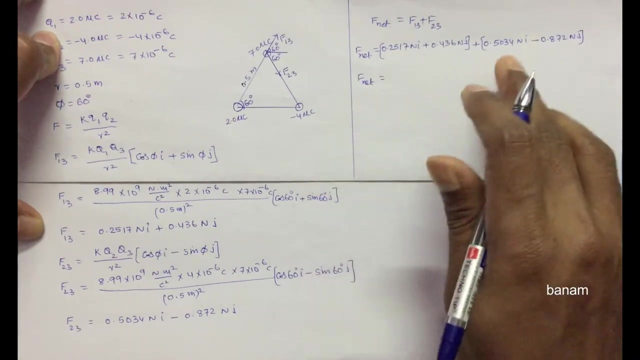 F13 is equal to 0.2517Ni bar plus 0.436Nj bar, plus F23.. F23 is equal to 0.5034Ni bar minus 0.872Nj bar. Fnet is equal to sum of the x component and sum of the y component. 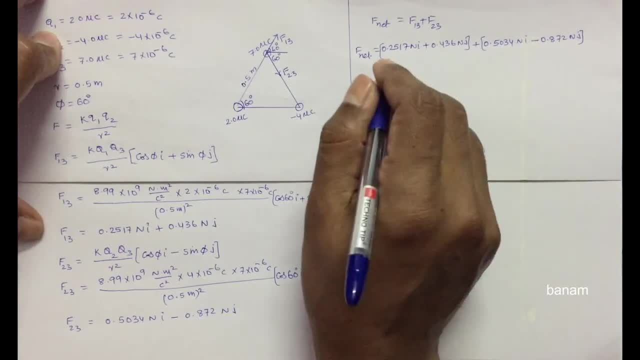 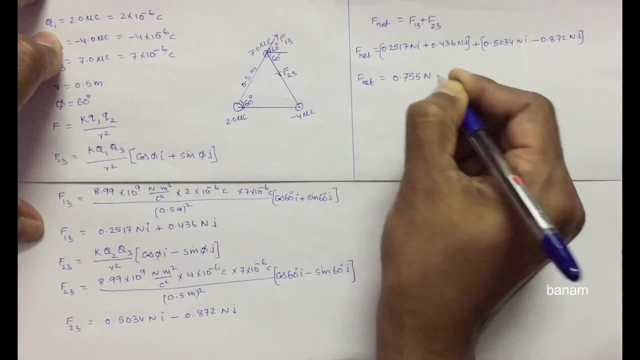 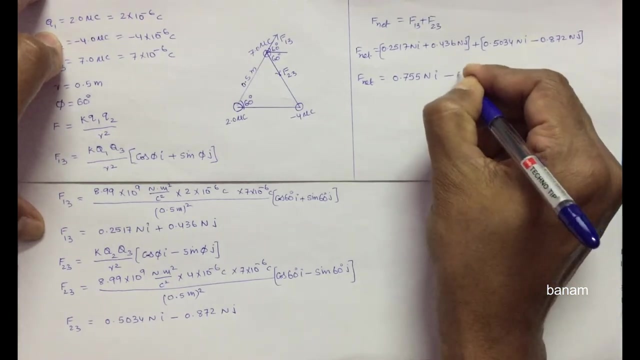 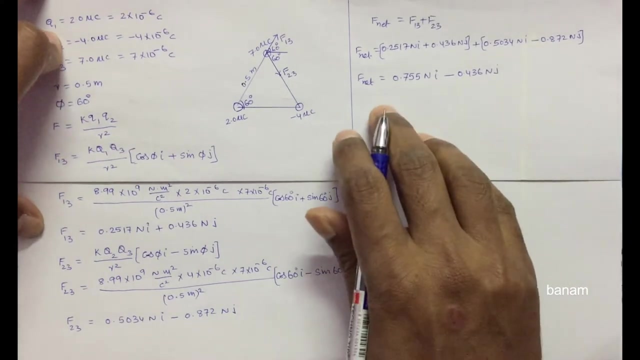 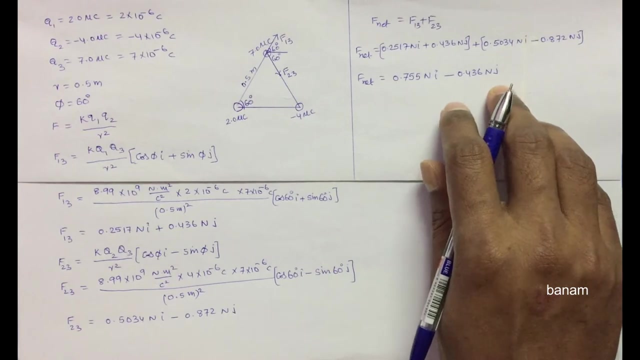 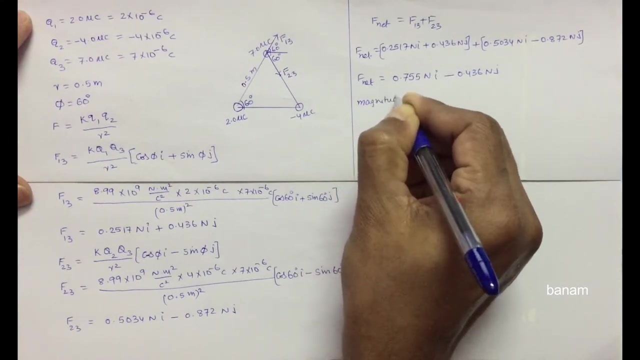 The sum of the x component is equal to 0.755Ni bar, minus sum of the y component, 0.436Nj bar. This is the vector component of the net force. The magnitude of the net force is equal to. magnitude of net force is equal to. 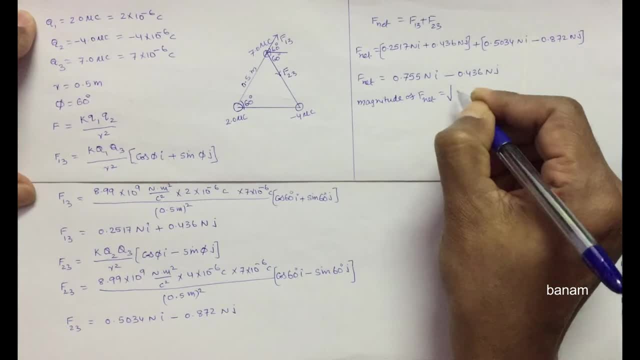 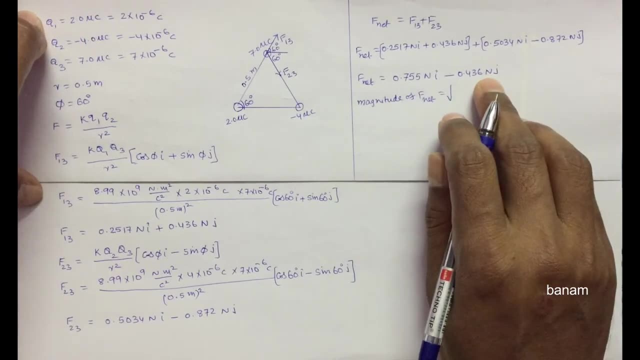 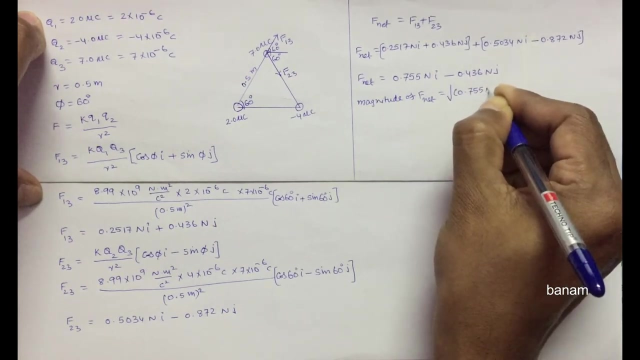 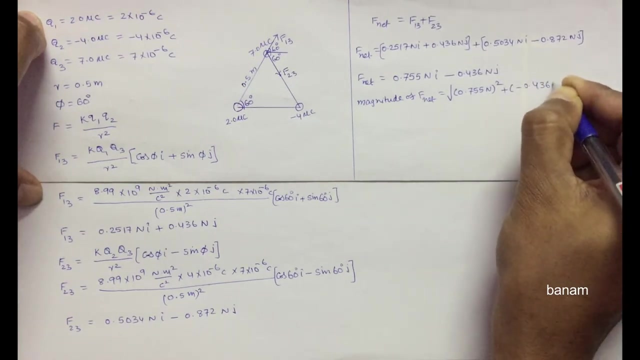 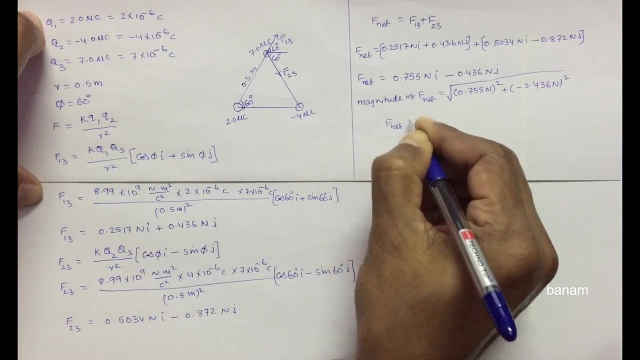 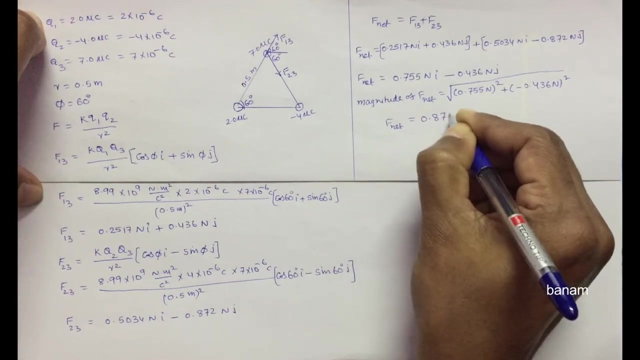 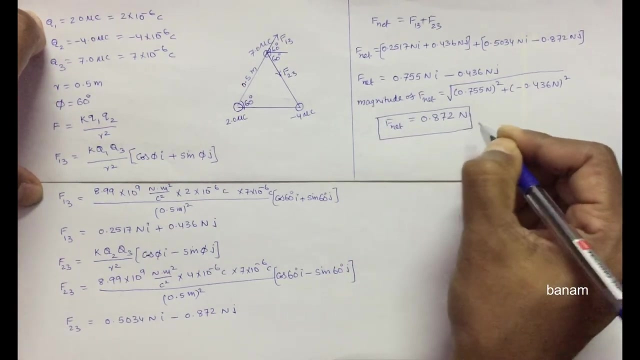 square root of square of the x component plus square of the y component, That is equal to 0.755Ni bar whole square plus minus cheesy 0.436 newton whole square. Fnet is equal to 0.872 newton. The net force on the 7 micro. 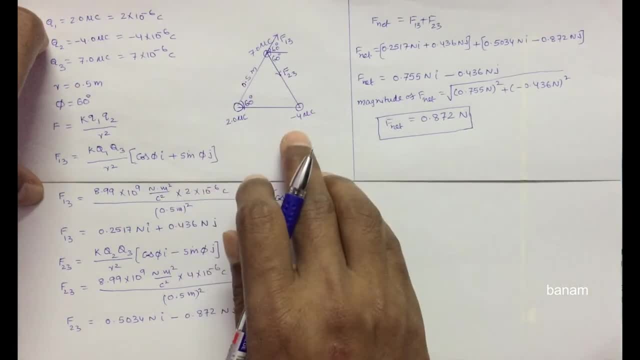 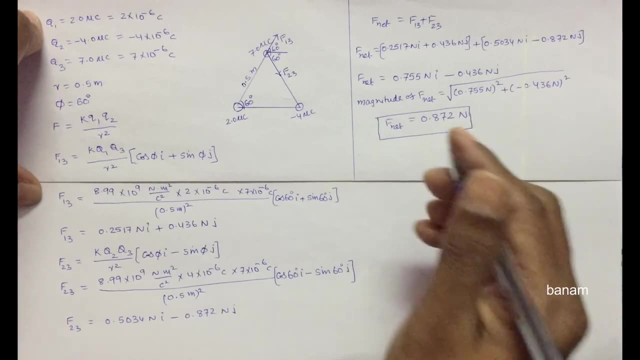 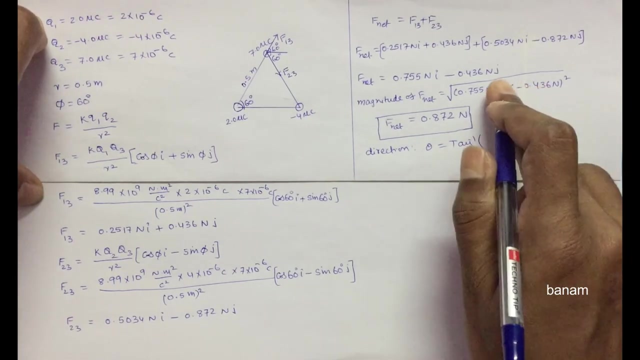 coulomb charge. due to 2 micro coulomb charge and minus 4 micro coulomb charge is 0.872 newtons. The direction of the net force. The direction of the net force. theta is equal to tan inverse y component of the net force by x component of the net force. 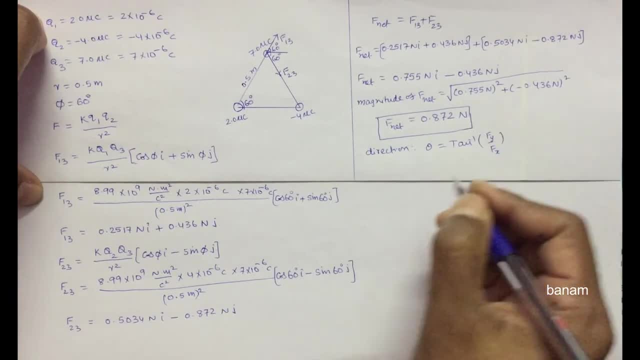 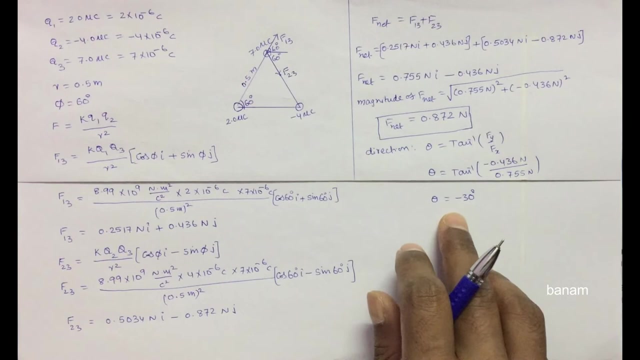 Fy. by Fx Theta is equal to tan inverse minus 0.436 newton y component and by x component 0.755 newton Theta is equal to minus 30 degrees. The negative sign indicates the the net force below the.